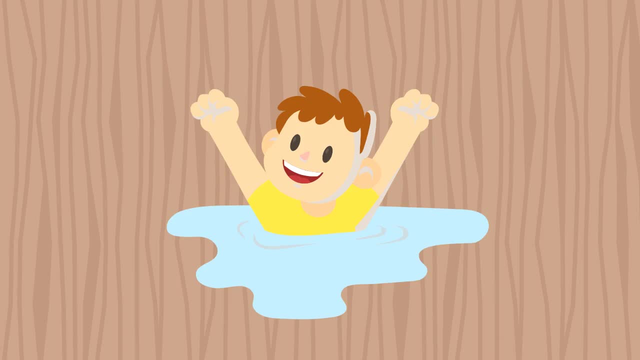 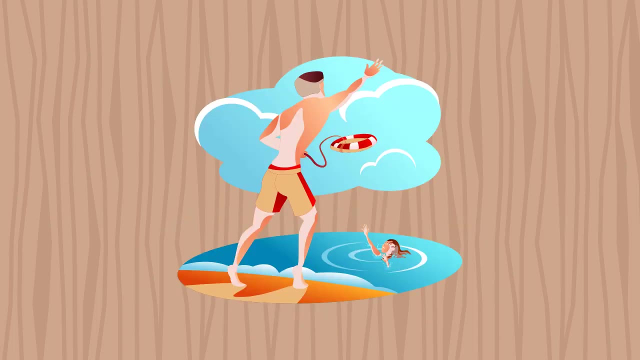 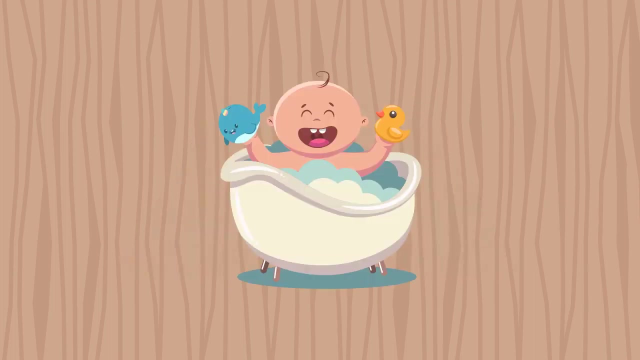 Hello and welcome to Pediatric Doctor at Home. Today's discussion is about drowning. Accidental drowning is one of the leading causes of death in children ages 1 to 4.. Drowning can happen not only in swimming pools, but in bathtubs, spas or any open standing water like ponds. 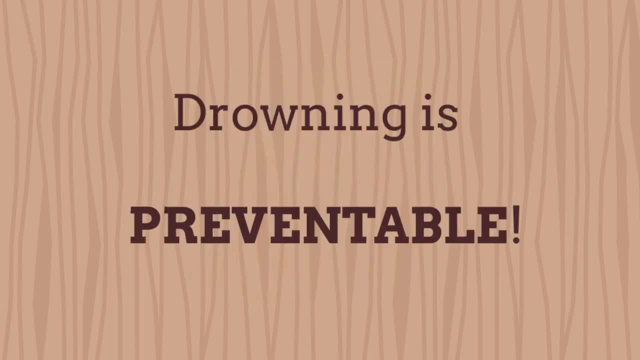 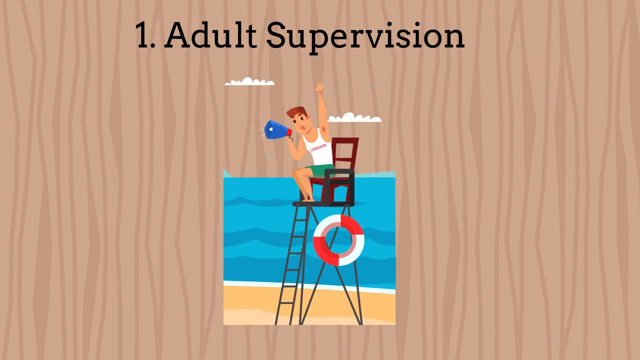 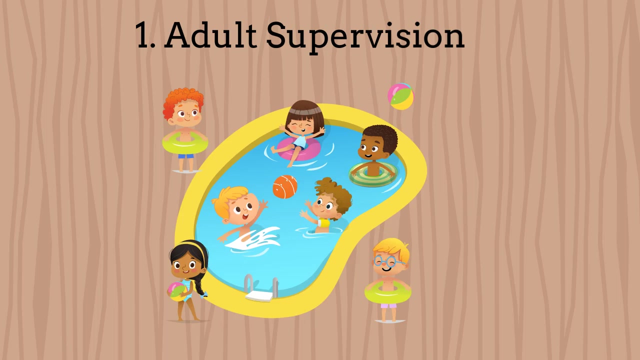 Tragic as it is. drowning is largely preventable, and here are 10 tips to avoid drowning in children. 1. Constant adult supervision. Never even for a moment leave young children alone or in the care of another child while in or around water. There must be a supervising adult. 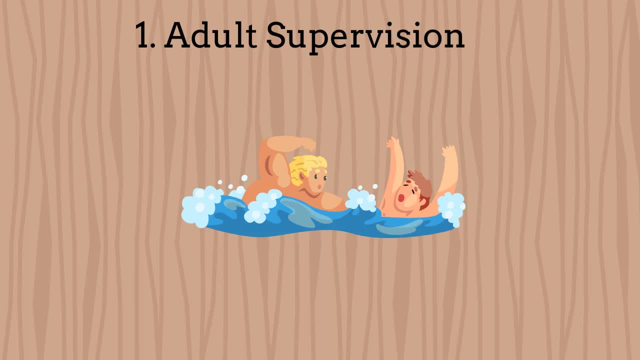 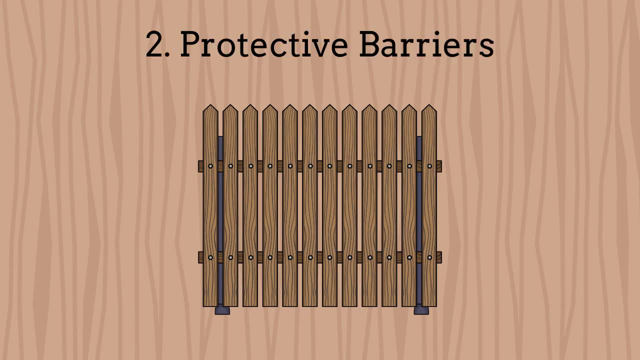 within arm's length, who is capable of swimming and not engaged in any distracting activity. 2. Restrict access to indoor pools using protective barriers or fencing. Install an isolation fence that is at least 4 foot high, with a self-closing, self-latching gate that. 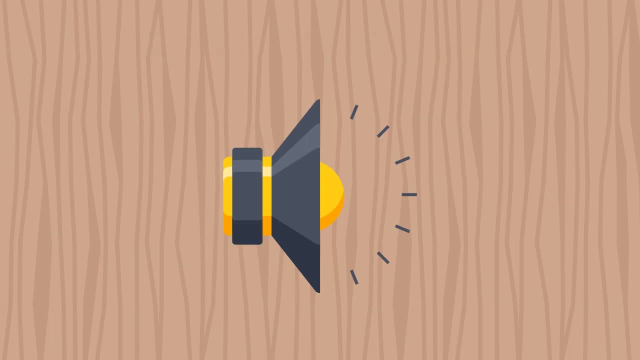 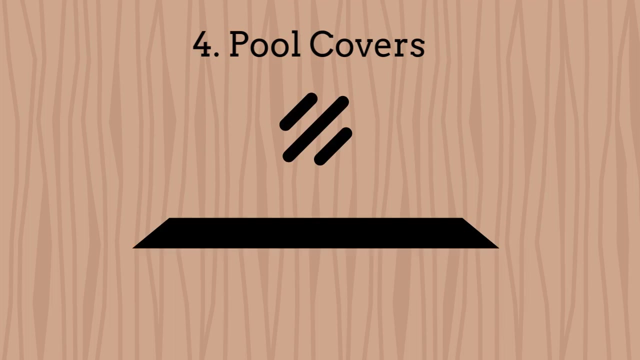 separates the pool from the house. 3. Consider purchasing a pool alarm system to detect and provide notification of entry into the swimming pool area. 4. Pool covers can prevent drowning. 5. Pool covers can provide an additional layer of protection. They must cover the entire pool. 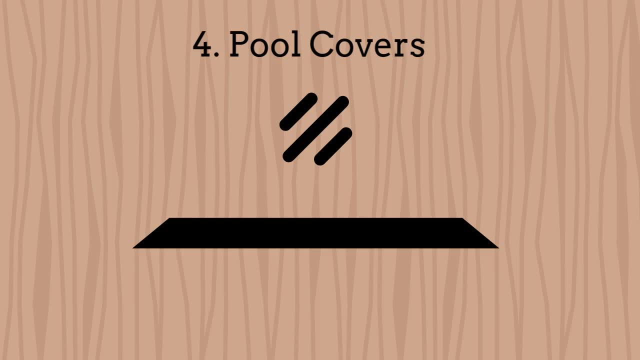 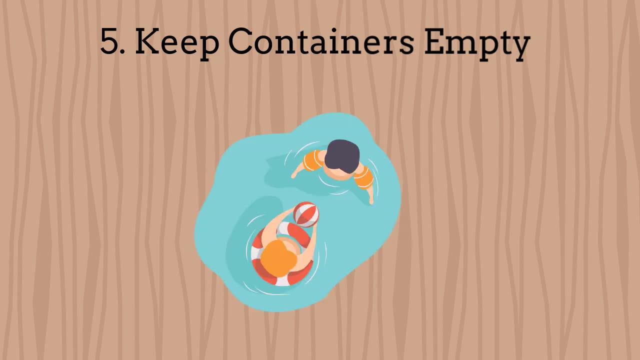 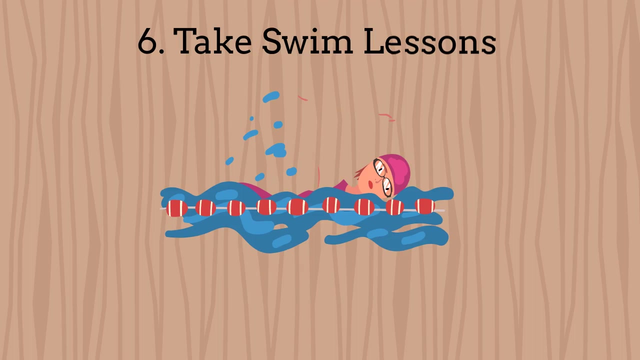 securely, with no standing water collecting on top of it. 5. Empty water from containers like buckets and inflatable pools immediately after use. 6. When available, children should take swim lessons until basic water competence is accomplished, Although swimming is not a guarantee against drowning at any age. 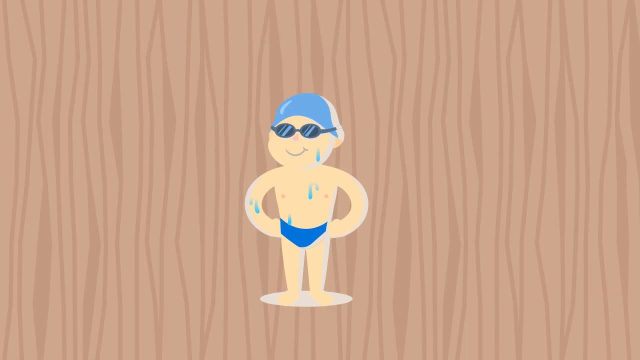 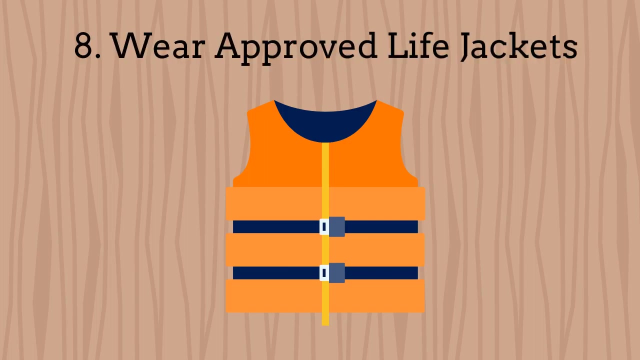 learning water safety skills is helpful. 7. Before jumping or diving, know the depth of the water. The first entry into water should be the feet. 8. Approved life jackets must be worn whenever required for water-related activities such as fishing, boating or water sports. Do not use equipment like inflatable arm bands, neck rings.